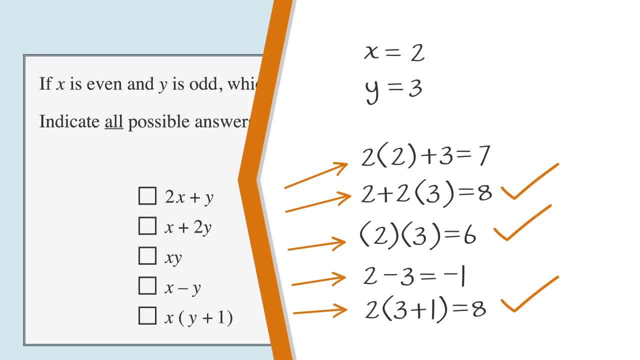 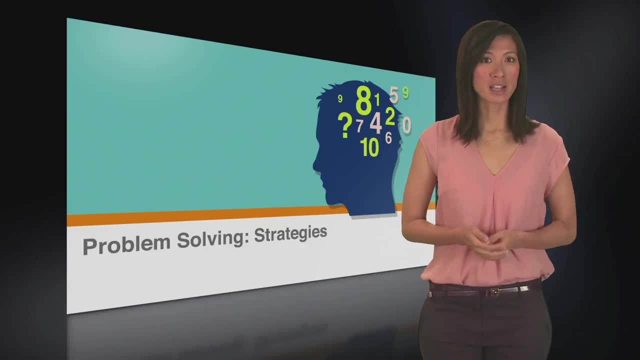 comes in handy here. So we check off the correct answer choices. Some problems, like the even and odd one we just saw, are more easily done by using the picking numbers strategy. Others are faster to do algebraically and the rest depend on. 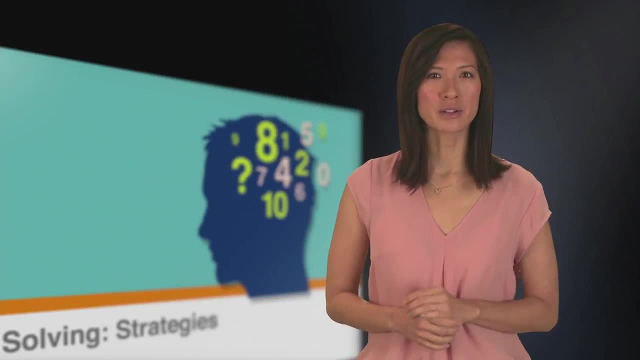 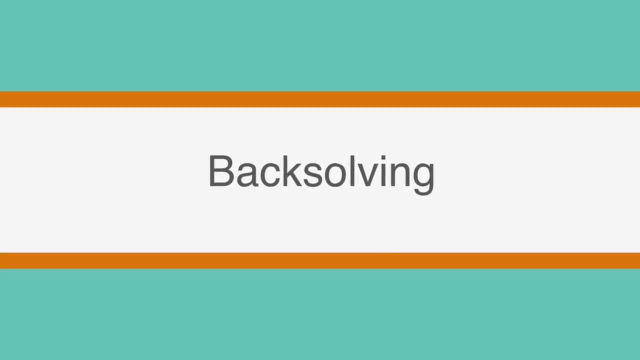 personal preference. The more you practice, the better an idea you'll have of which strategy works best for which kind of problem. Now let's look at back-solving, another strategy that can be used with our problem-solving method. Back-solving just means to pick a number that fits the question and pick an. 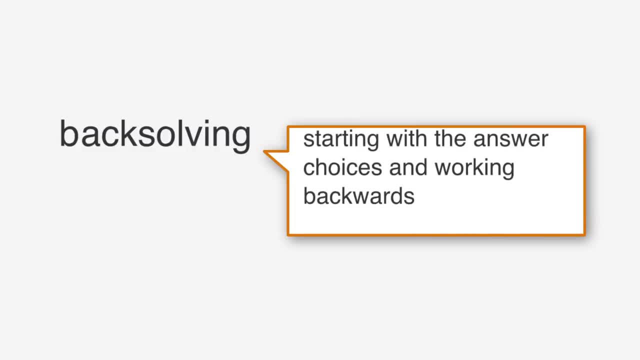 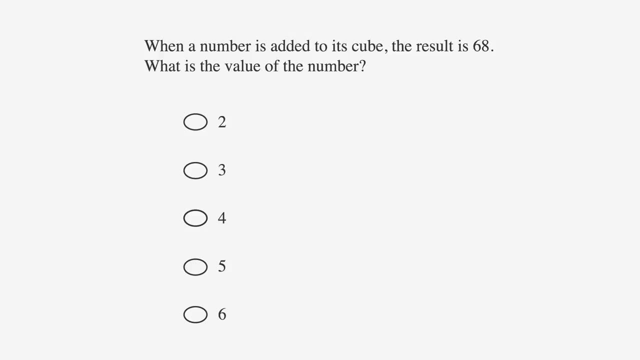 answer. Back-solving just means starting with the answer choices and working backwards. Let's try our new strategy on a problem When a number is added to its cube. the result is 68.. What's the value of the number? The answer choices are 2,, 3,, 4,, 5, and 6.. 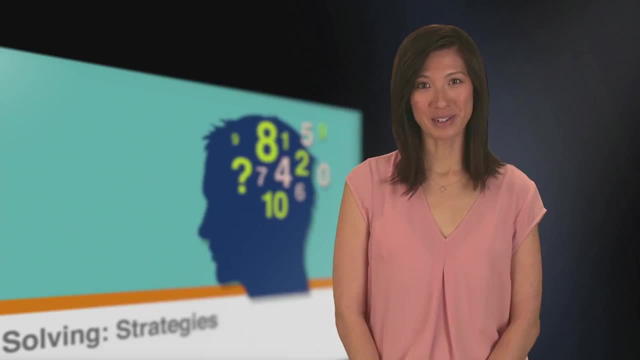 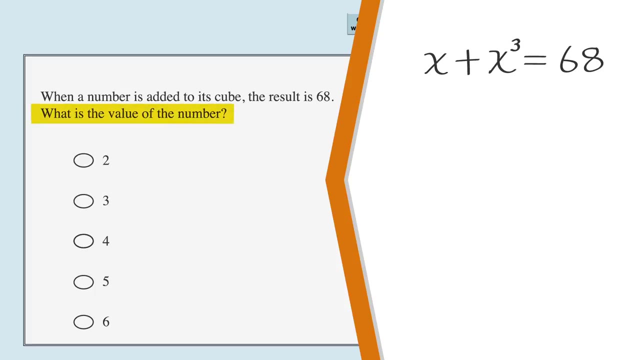 Keep in mind that the cube of any number is that number to the third power. First rewrite the problem mathematically. We have X plus X to the third power equals 68. We're then asked for the value of X. Next, back-solve for the answer choice that gives us 68.. 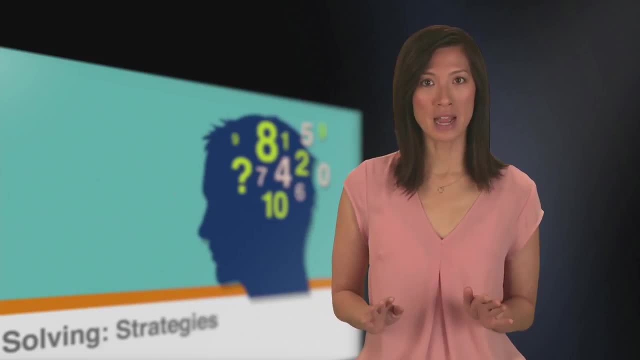 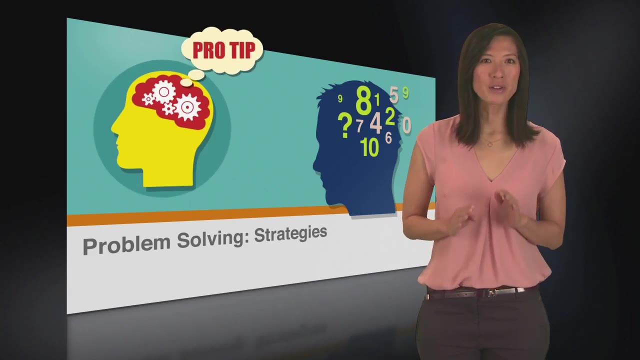 When we back-solve, we need to have a process. You will never have enough time to solve for every option, so we'll try to go over the most time-efficient way. Here's a pro tip for you All: numeric answer choices in the quantitative reasoning sections. 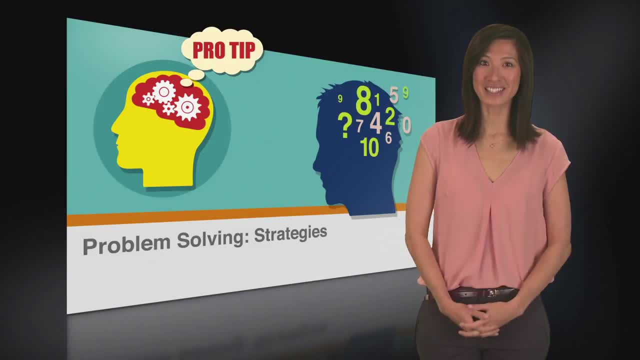 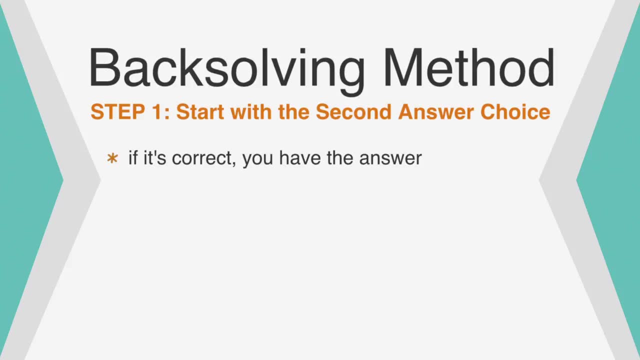 are listed in increasing order, So let's take advantage of this. Step 1 is to start with the second answer choice. If it's correct, you have the answer. If the input is too large, the answer is wrong. If it's incorrect, you have the answer. 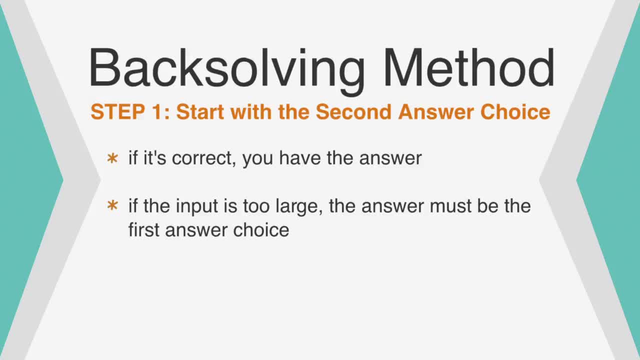 If it's too large, the answer must be the first answer choice, because the first answer choice is smaller. If the input is too small, that means the first and second answer choices are too small and you can eliminate them both, Since we can determine if the first and second choices- 2 out of 5, are correct or not. it. 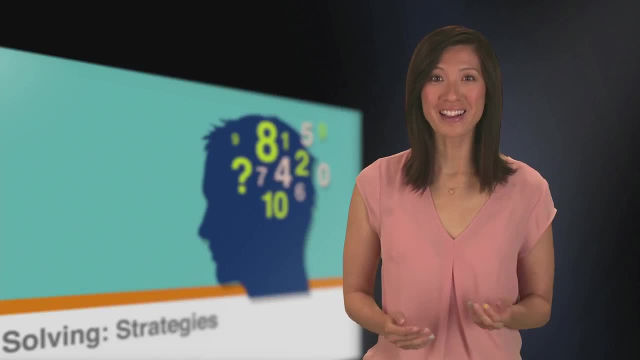 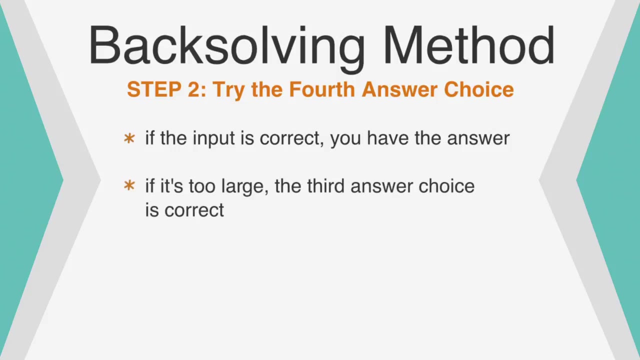 means we have a 40% chance of finding the answer on the first try. Step 2 is to try the fourth answer choice. If the input is correct, you have the answer. If it's too large, the third answer choice is correct. 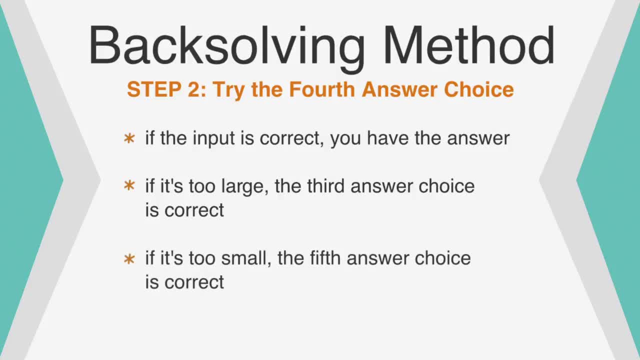 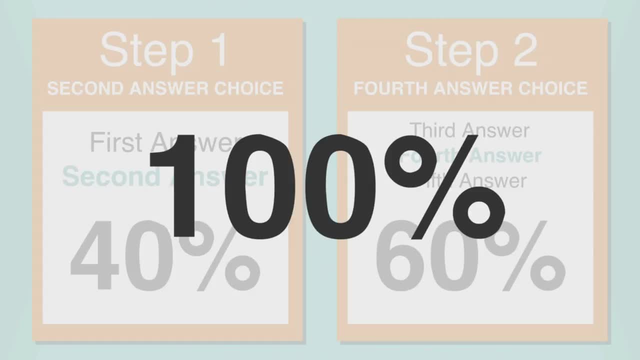 If it's too small, the answer must be the fifth answer choice, Since Step 2 determines which of the remaining three answer choices is correct. we have a 100% chance of finding the answer in only two tries, Testing all five answer choices.